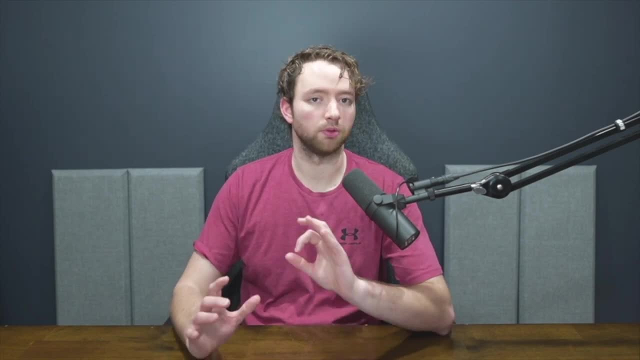 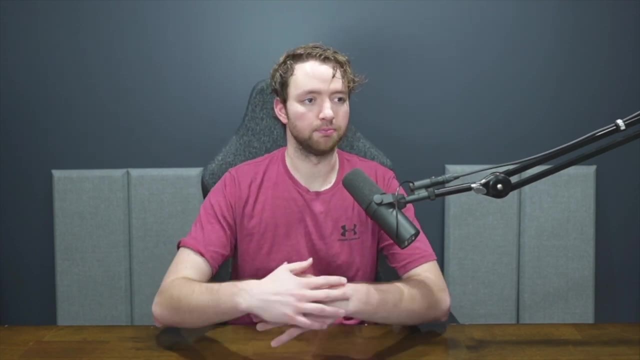 going to go through a fairly simple example, and you should try to understand this material before moving on to the next video. So you start by creating what's known as a class. This is a blueprint, a structure that basically describes what something would look like. The 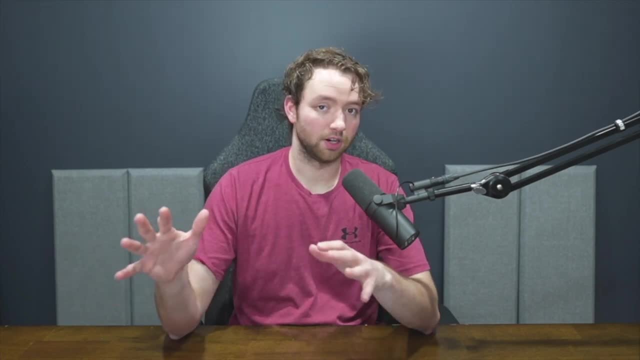 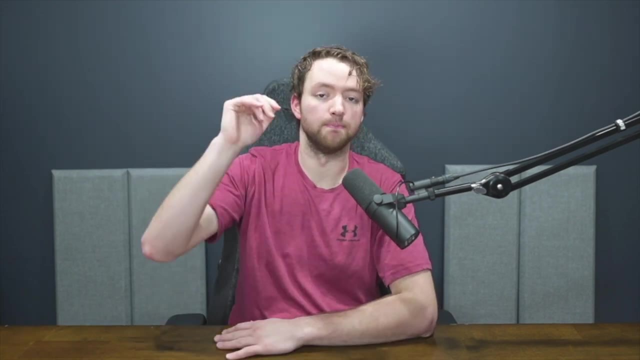 class is then instantiated- Fancy word- And this means we create something also known as an object based on that structure. So we have a class and then we can create multiple objects from that class. So here we are in our code. We still have some functions from earlier, but we're not going. 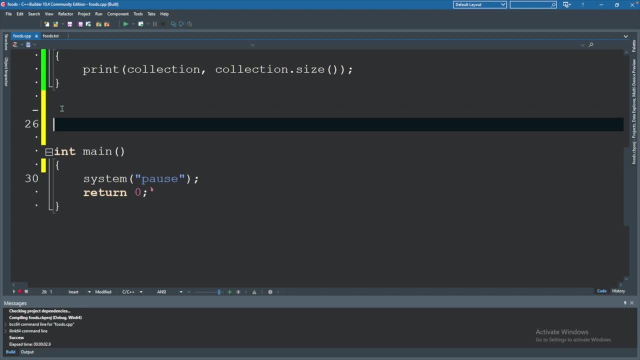 to need those right now. So don't worry about it if you're just jumping in for the object-oriented programming content. What we will do is we will define a class and describe some concept, such as food, And then you will have curly braces And note there's no. 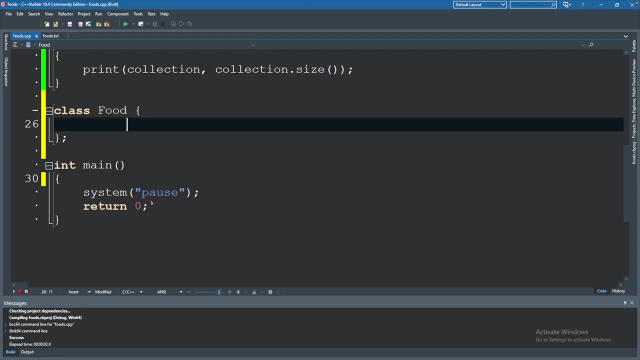 parentheses, like you normally define functions or if, statements or anything like that, And inside of here you're going to have the keyword public And then inside of this, after a colon, is where we're going to define what a food looks like, So it can have different data attributes, such as a. 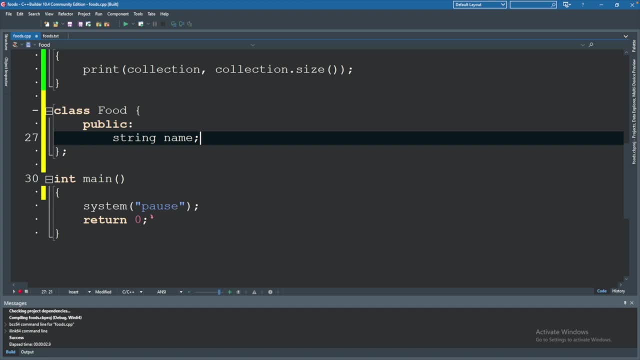 name, what the name of the food is, like banana, Whatever other foods there are. Literally can't think of anything And you can have any data you want. So let's say you were keeping track of the cost of all these foods you're buying from the 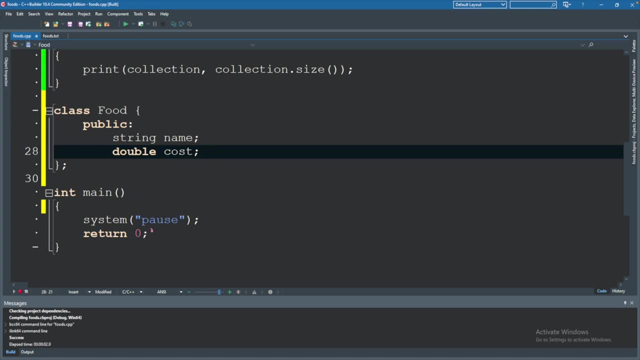 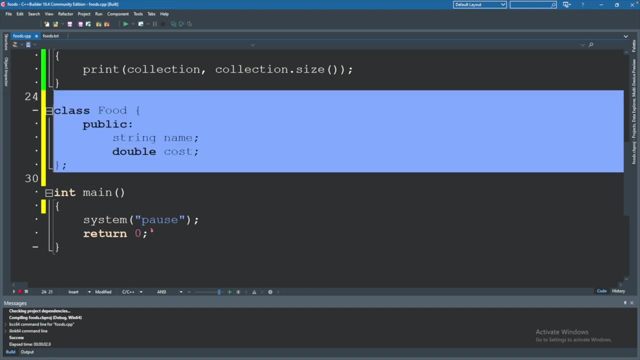 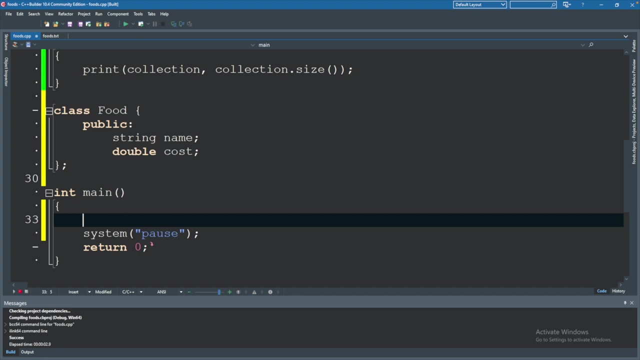 store, You could have a double cost, Double being just a number with a fractional part, So $10.15.. Now this is the class. We're not actually making a specific food To create a specific food that's known as an object, And we can do that inside of our main code, So we will do that here. 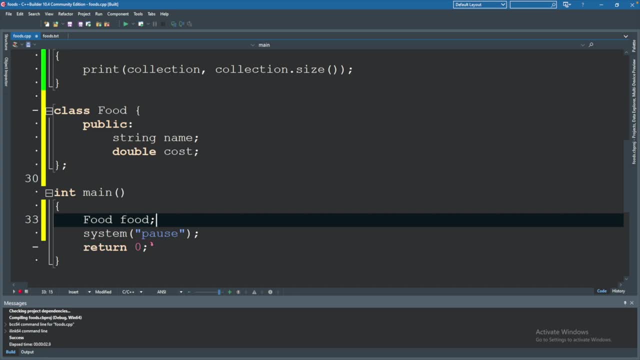 You will say what type the variable is And then give it a name. Now I'm going to name these, both food- One lowercase and one uppercase- And people sometimes get annoyed that I do this, but I do this on purpose, because it's convention. 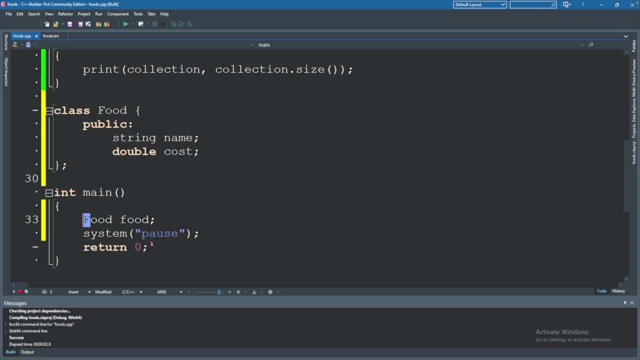 The lowercase refers to the variable. The uppercase refers to the type. There's no need for you to have different names for these. You should be able to look at these and just know what they are. So what I mean by type is we're actually creating a custom type here, Just like we could create a. 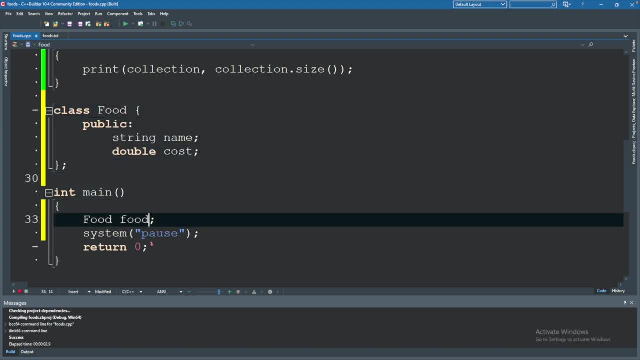 string or a double. Now we can create a food- Pretty cool- And the food can have different attributes. So food dot is how you access those different attributes And you can say name. Give it a name, such as bananas And food dot cost. 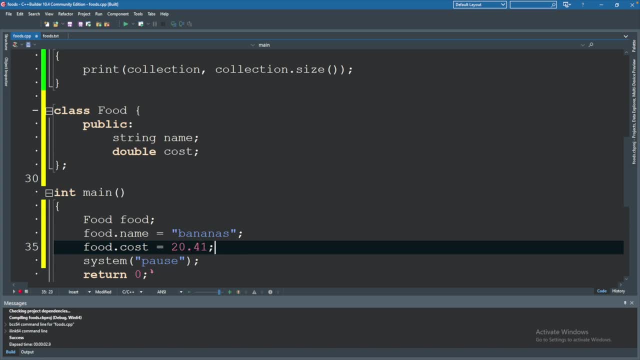 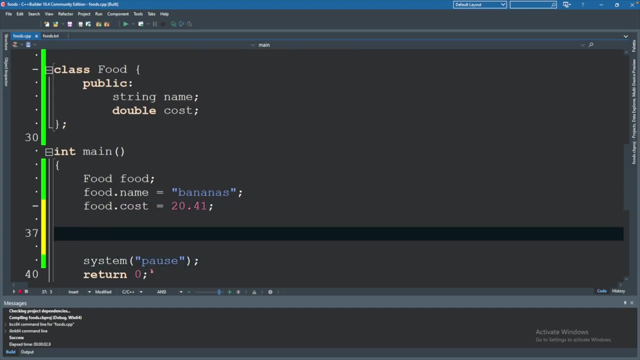 Give that a value such as $20.41.. Pretty expensive bananas, but inflation right, All right. So now how do we actually access these values? We'll say cout, food dot name And let's go to space, And then food dot cost, End L. We'll run this And you can see it says the food name. 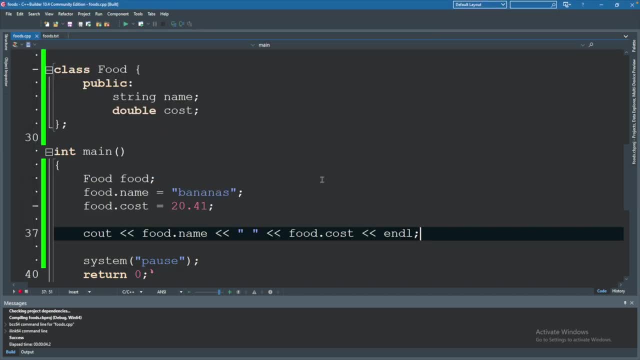 and then the cost. So it's basically a way to organize data And it makes sense when we have a bunch of data around a certain thing, such as a food, So we can have data members like these here which store some data, But we can also have methods which will do something, So we could say: 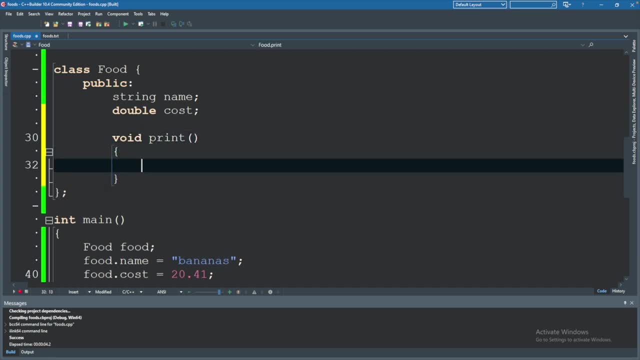 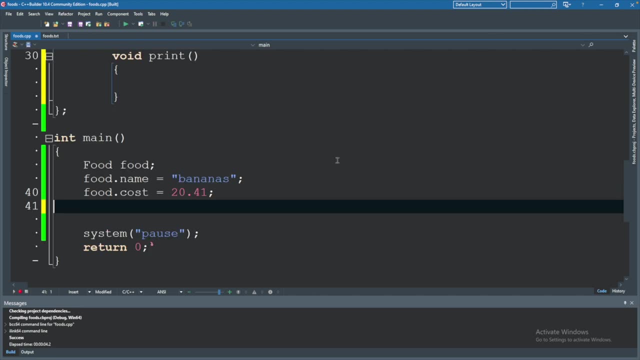 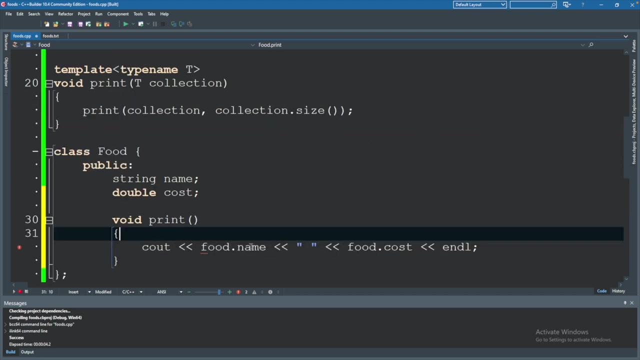 void print, And this can be used to print all of the data. So let's just go ahead and copy This example here, But we're going to have to modify it a little bit, So I'll cut that from there and paste it here. Clean up the formatting just a bit. You can see this food here now, doesn't? 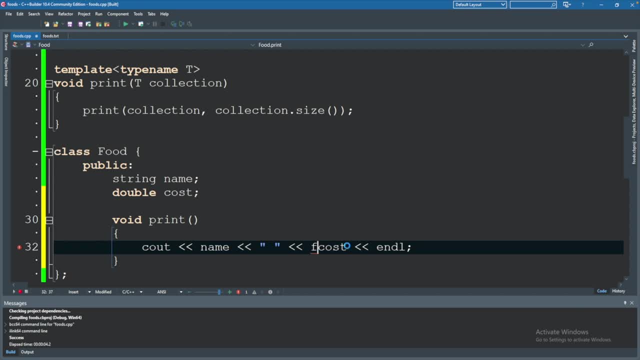 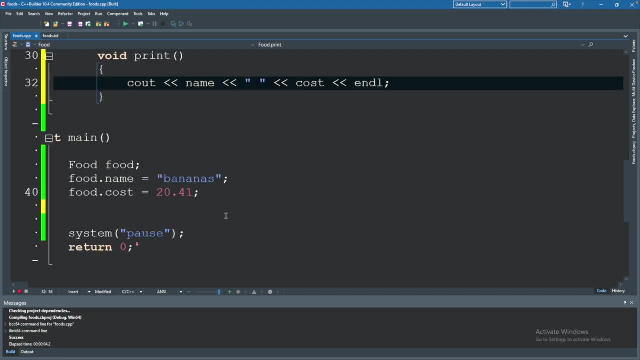 exist. We can actually just remove that And it knows what we're talking about. It's going to refer to whatever object we're currently invoking print on. So to use this, we will just say food dot print. Let's run this and confirm that we get the output we would expect. 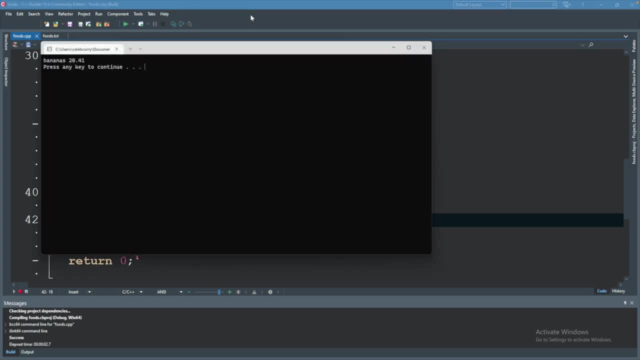 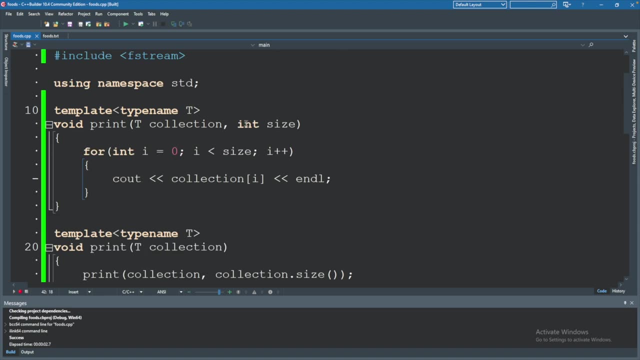 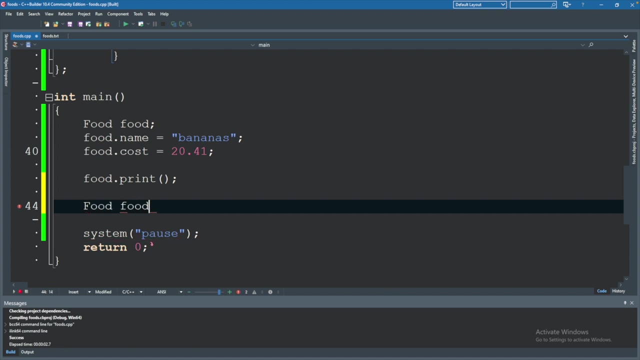 And there we go. We get the same exact thing, But since this print is related to the food, it just makes sense to put that inside of the class here. The cool thing is now we can create multiple foods. So if we wanted to create another food, we could say food two, And then we could say: 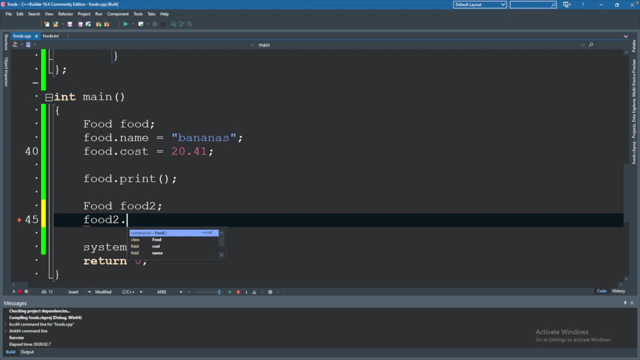 food two. Make sure you have the two so you're not changing the other food name And we'll go with something like cheese and food two. So we'll go with food two. dot price, I don't know, $274.. My bad, I got the attribute name wrong. So